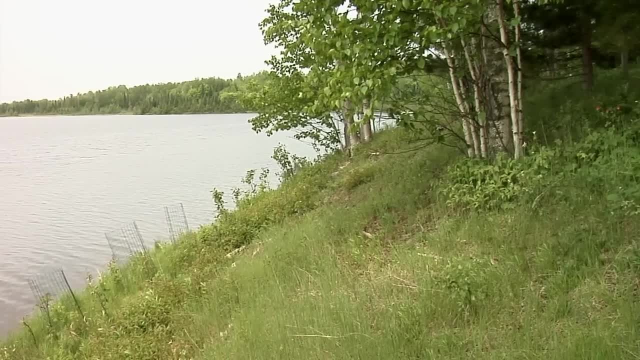 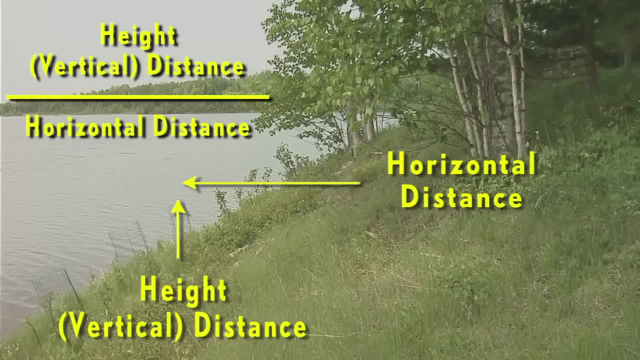 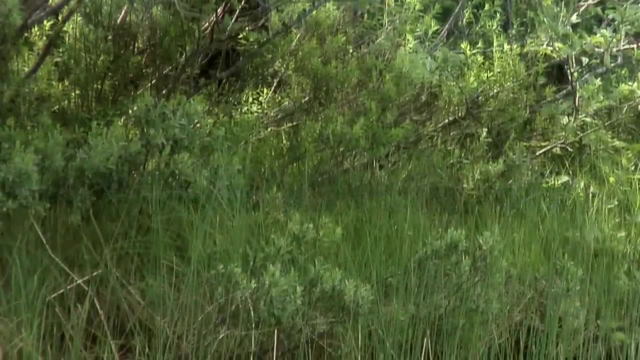 to runoff and erosion issues. In simplest terms, slope is the change in height over a horizontal distance. This simple formula is often expressed as rise over run. Multiplying this value by 100 converts it into a percentage. Slopes of 6% or less are of relatively little concern, although 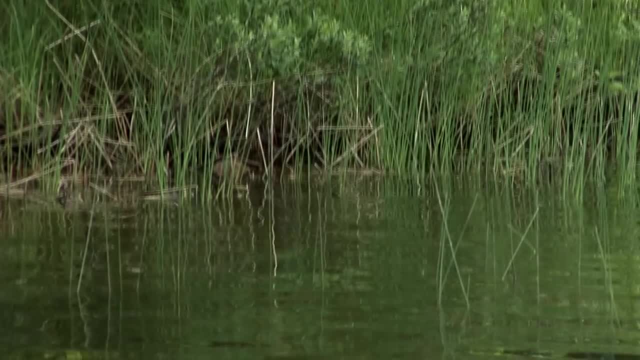 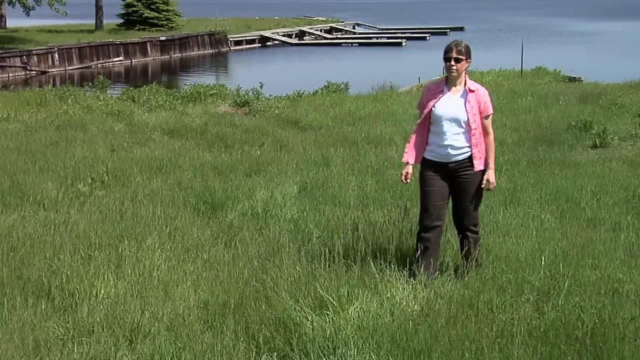 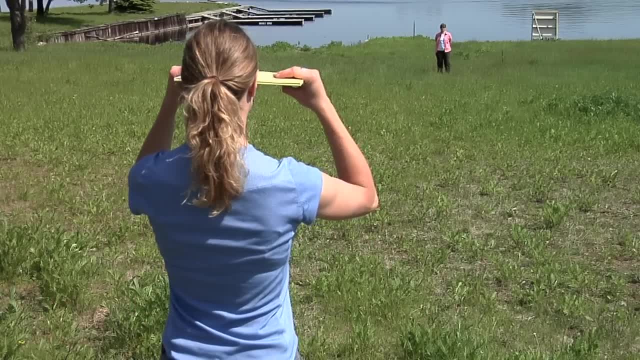 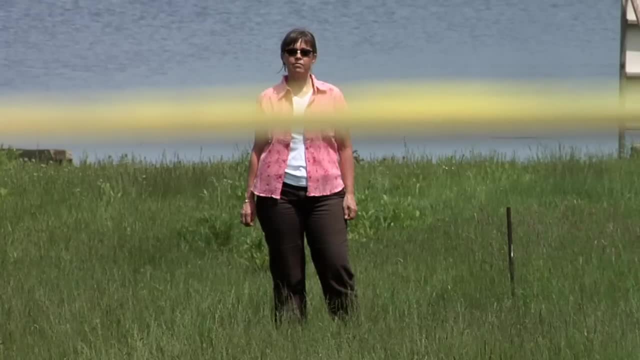 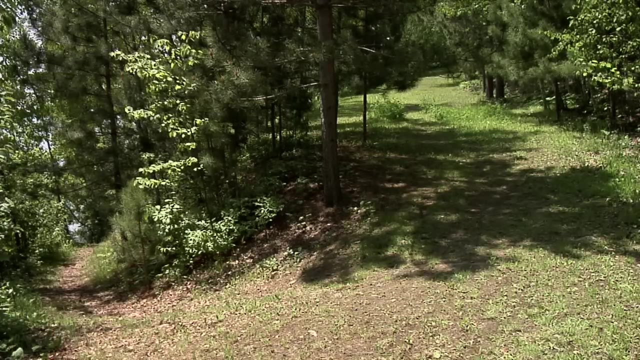 Using a notebook or another flat surface to block anything below the horizontal sight line. if the person on the uphill side can still see any part of the downhill person's body, then the slope is most likely less than six percent. If you estimate that your slope exceeds six percent, 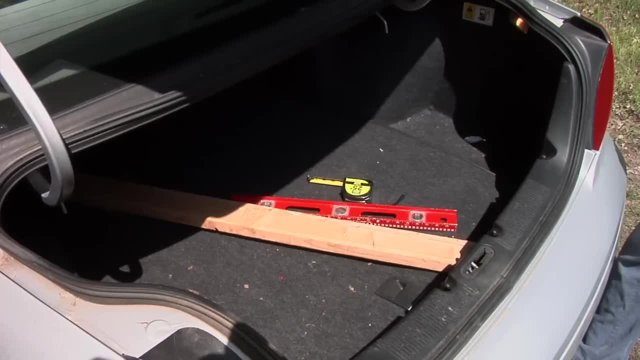 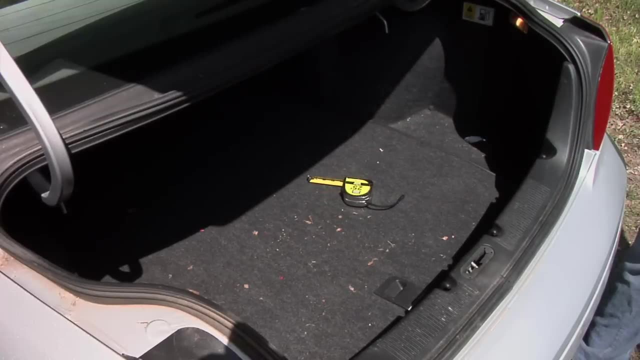 a more precise measurement will be needed. There's a simple way to determine this: using a few common items and some easy math calculations. You will need a 50-inch board, a carpenter's level, and a tape measure. Place the board flat on the ground at a. 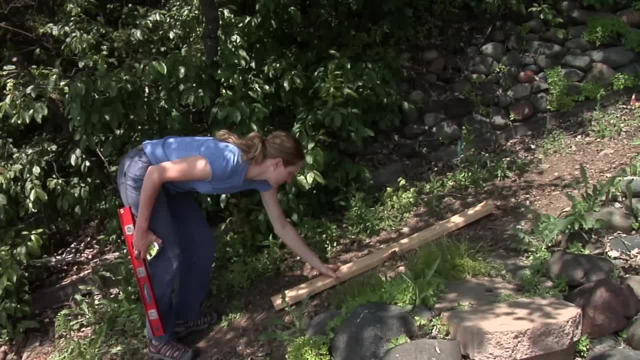 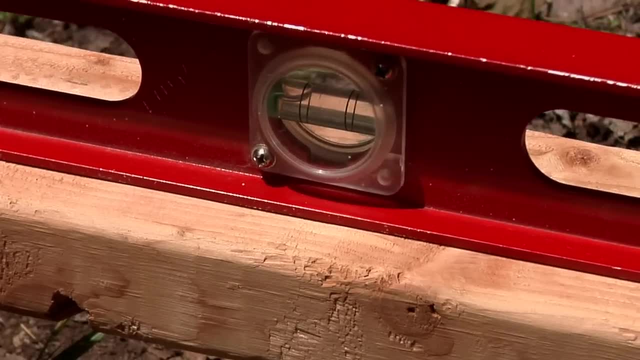 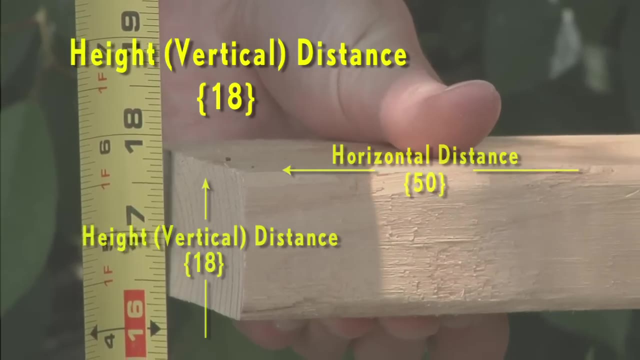 good representative location, with the length going up and down the slope being measured. Set the level on the 50-inch board and lift the lower end of the board up until it is horizontal. Now measure the plumb line distance in inches from the raised end of the level board to the ground To determine the slope. 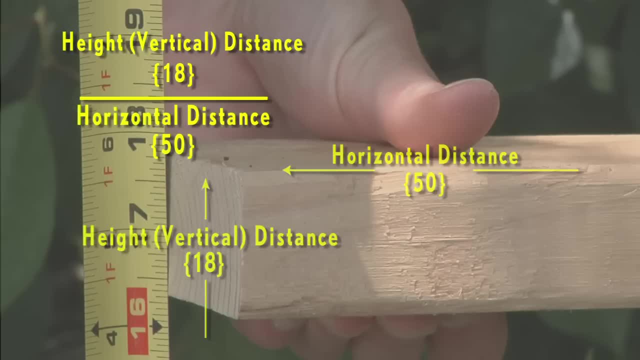 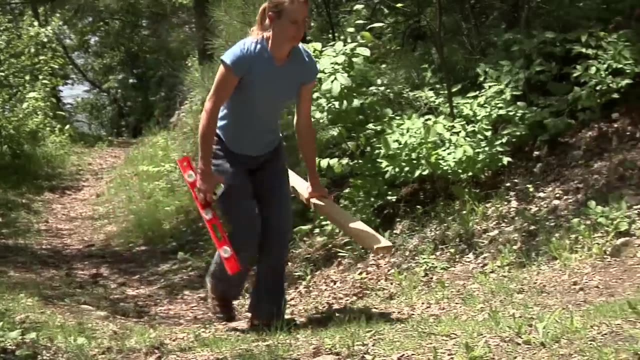 divide this number by 50, the length of the board, then multiply by 100 to express this value as a percentage. To ensure the most accurate measurement of slope over the whole area, you should repeat these steps at several different spots that are representative.